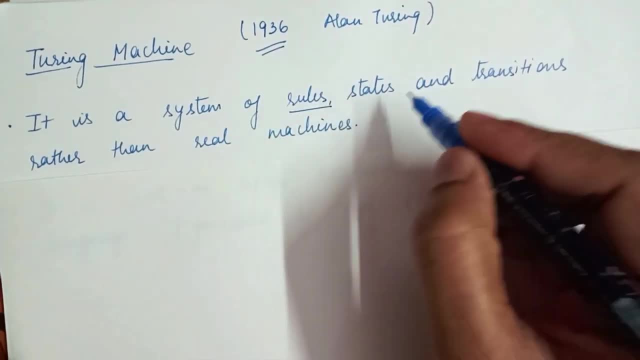 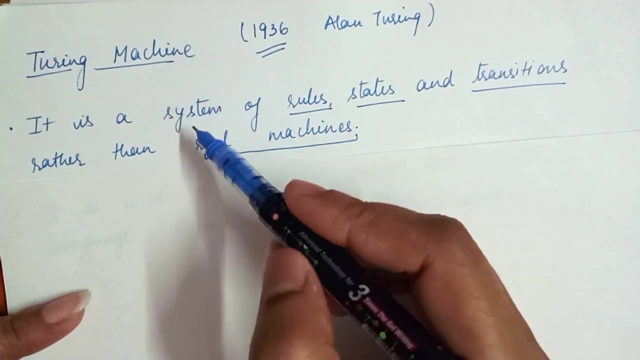 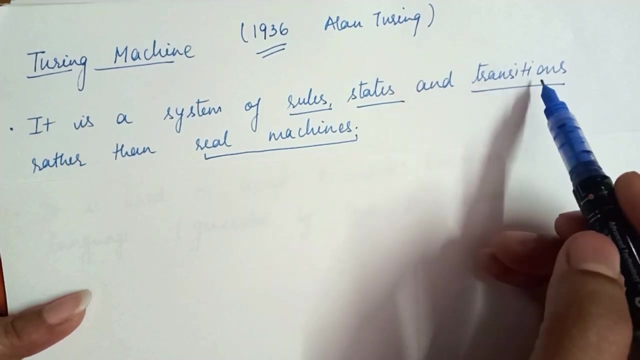 then it is a system of rules- okay, states and transition, rather than the real machines. so a turing machine can be defined as a system. we define some set of rules, some states and the transition between the states, rather than some real machine. okay, and the two? there are two. 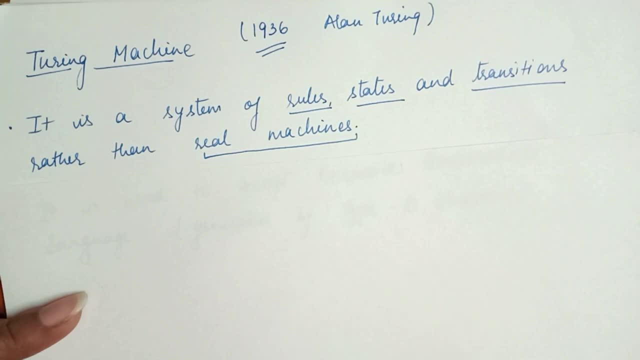 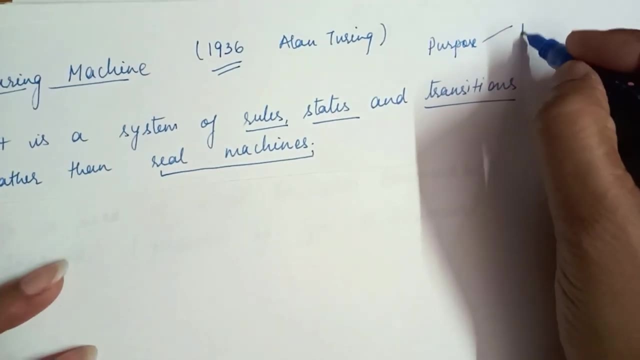 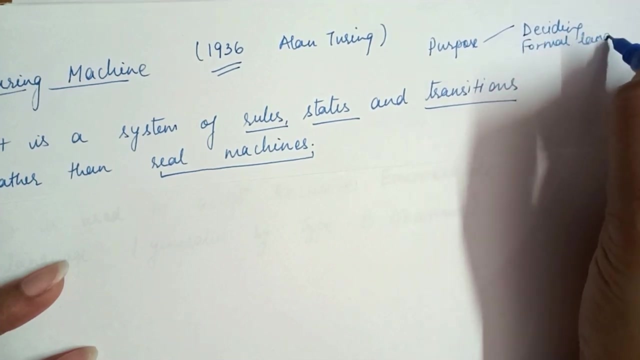 purpose for which a turing machine will be used. the first purpose is: so there are two purpose that either aandez is using or cibi or other turing machines. so the purpose that正 색 is former language. so when we are using a turing machine, the first purpose we use is: 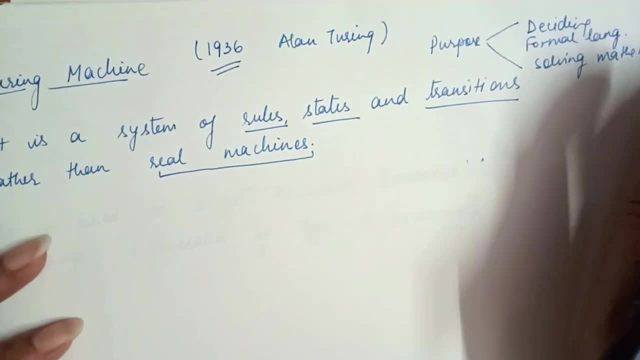 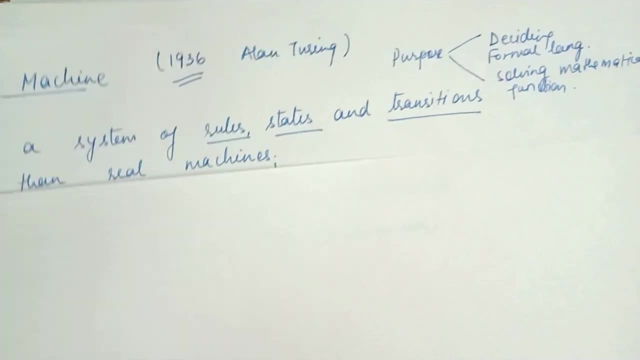 we use uh cibi calculation for a problem in the wir scenario that the turing machine can be used, and the second we use parsal vitamin. we can also using other terms, we use means also, we sometimes us- and then we can also solve, so that this problem can be solved by us. we can also solve by also civil language. 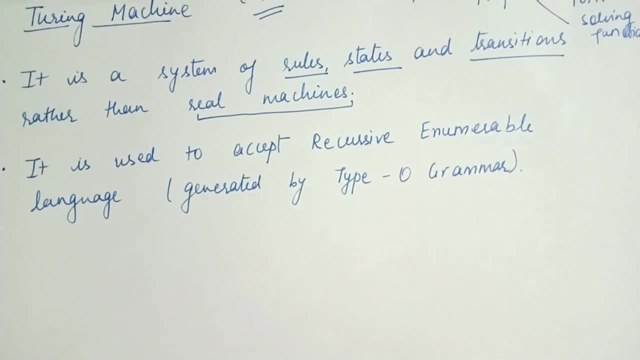 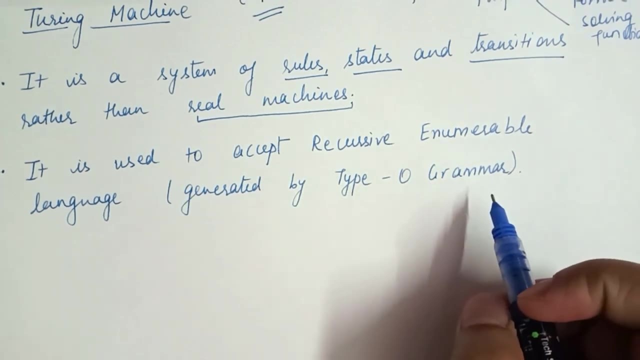 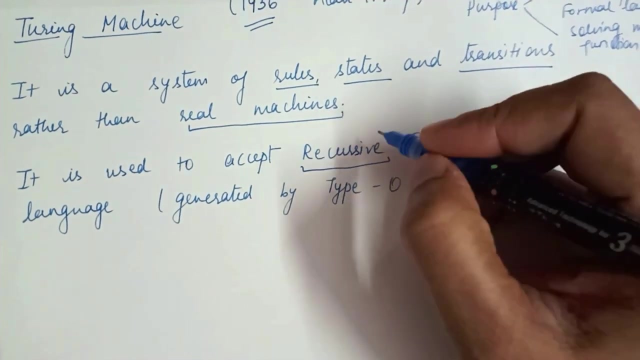 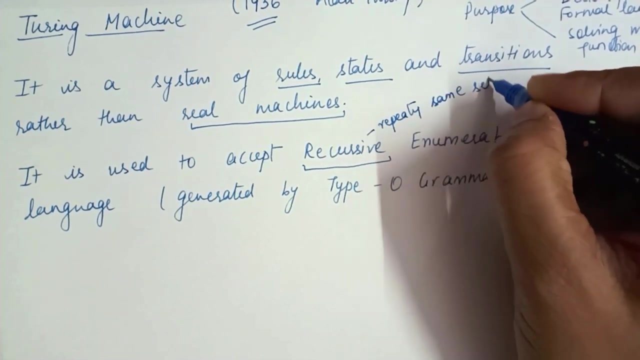 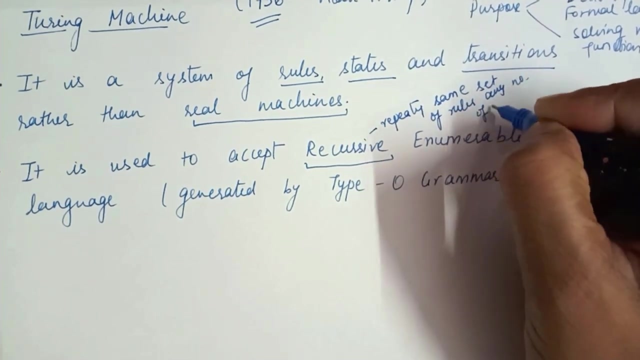 So it is also used to accept recursively enumerable language, and this recursively enumerable language is generated by type 0 grammar according to the Chomsky Grammar. So this recursively enumerable grammar language means recursively means repeating same set of rules, repeating same set of rules any number of times. 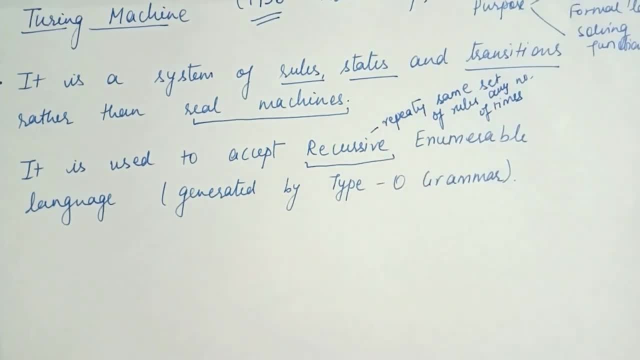 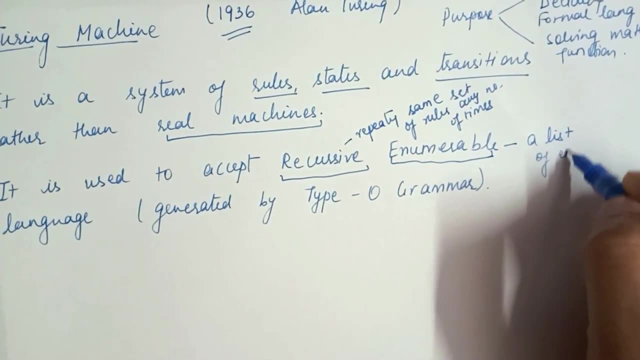 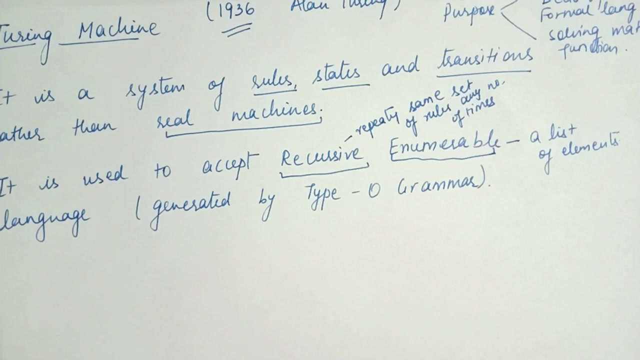 Any number of time. this means recursive and enumerable means. this enumerable means a list of elements, a list of elements. So this Turing machine it is used to accept this type of enumerable language, which is also known as type 0 grammar. this Turing machine is a most powerful machine to which can be accept any type of languages. 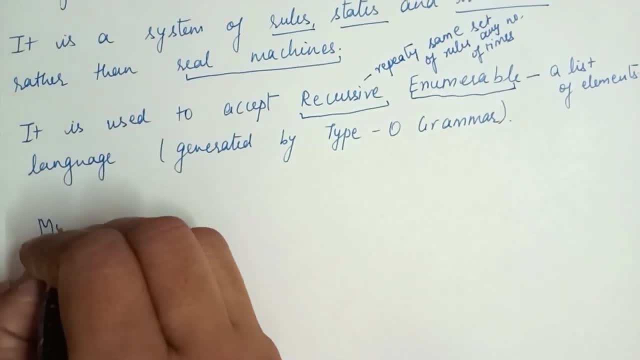 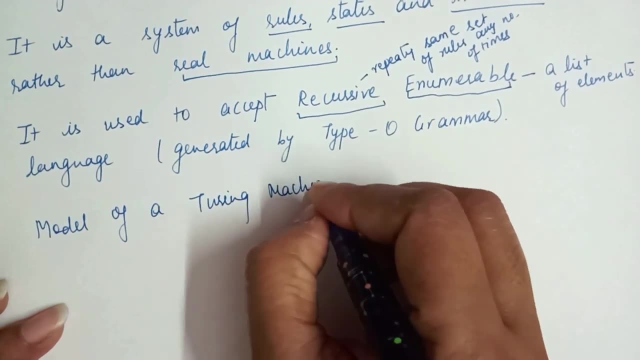 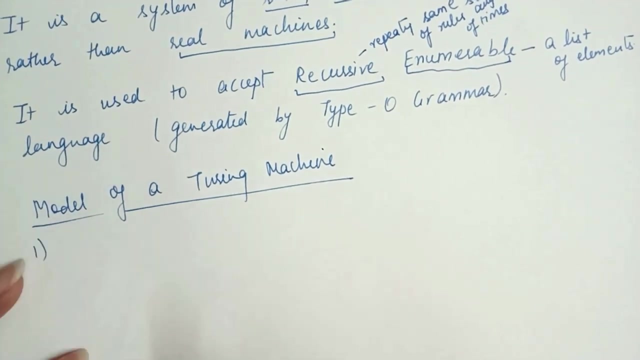 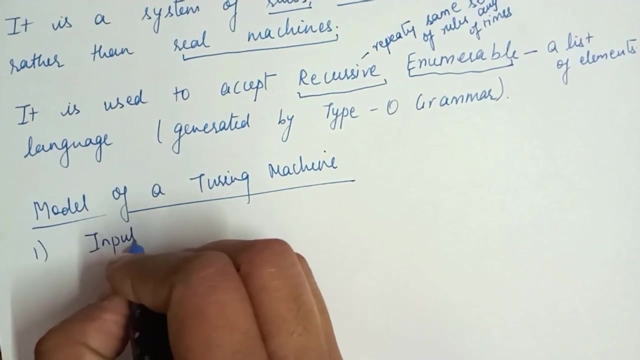 Okay. so if we talk about the model, the basic model of a Turing machine, model of a Turing machine, then it can be modeled with the help of the following representation. So the first representation will be: that is input tape, input tape. So the first model of a Turing 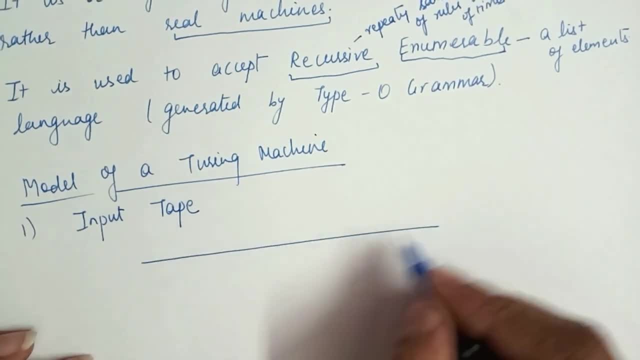 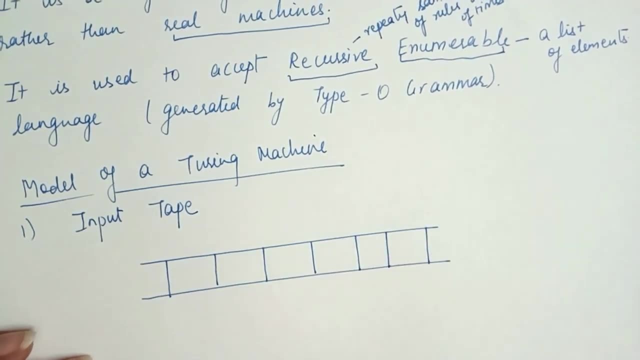 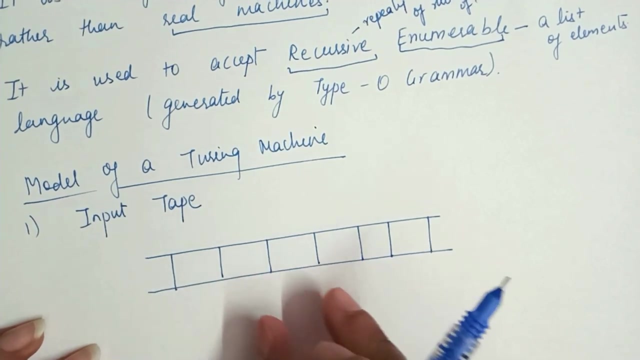 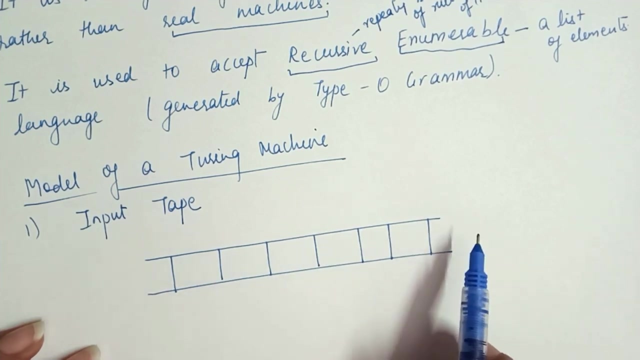 machine is input tape. This input tape can be represented by like this, like this: Okay, so the input tape is having a infinite number of cells and each cell containing one input symbol, And thus the input string can be placed on this tape and the empty tape is filled by. 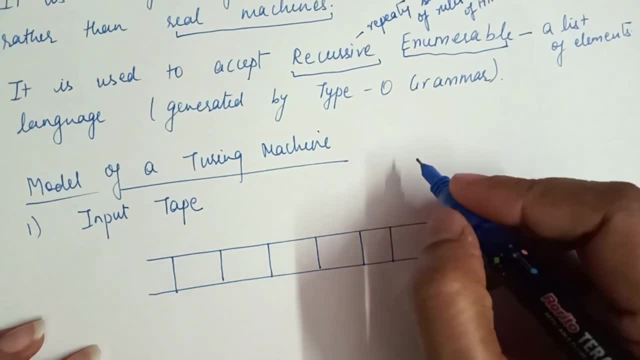 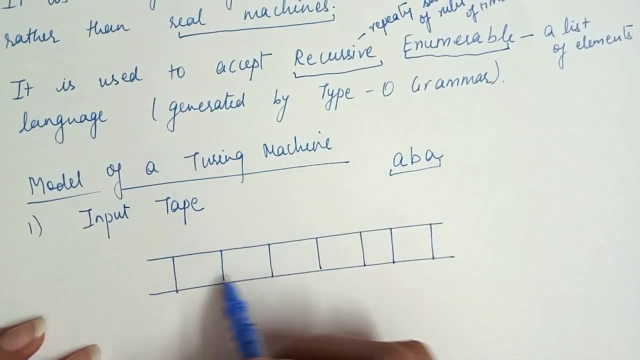 a blank character. Suppose if we have an input string- ABA. Okay, so this input string or input symbol is filled into this input tape, like this ABA, and the remaining empty tape is filled by some empty character, blank character, which we denoted by ABA. So this: 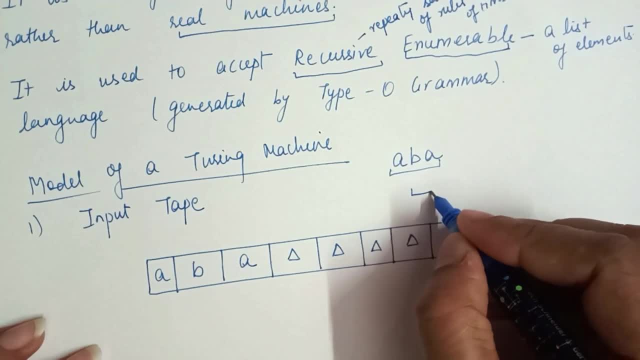 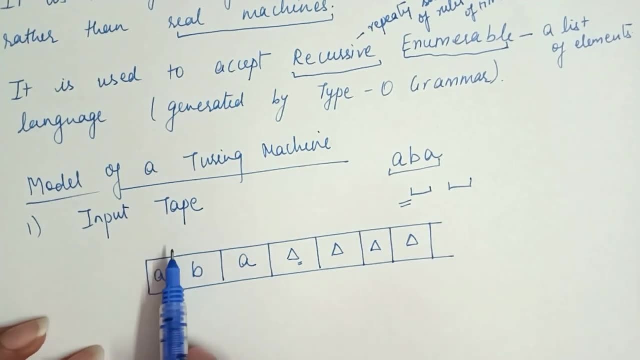 input type is called the blank type. that is filled by delta And in some book the blank character is noted like this: so you can use this. or either you can use this, So this input tape, the first component of the Turing machine is the input tape, So this input. 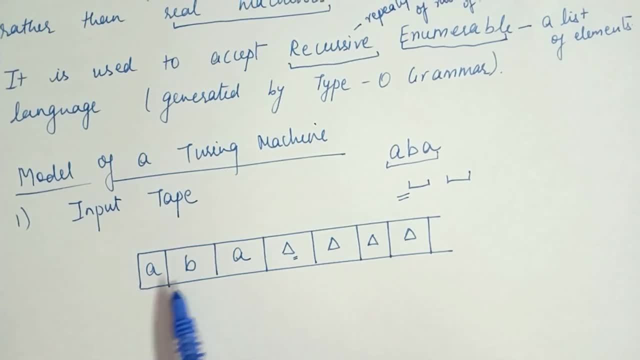 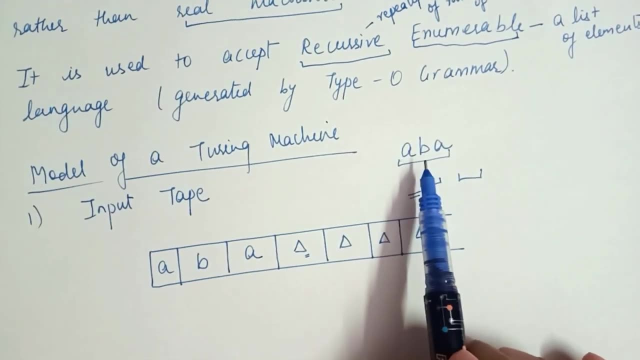 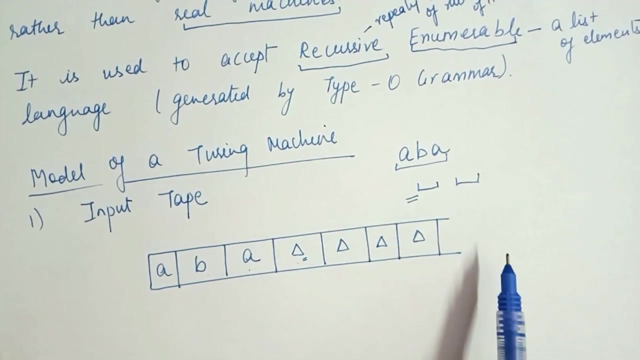 tape is having an infinite number of cells and in each cell we contain a set of one input symbol and thus this input string. like this, For example: if we have an input string ABA, so we fill ABA, BA, and the remaining we will fill by the blank character. Okay, so this is the first component. 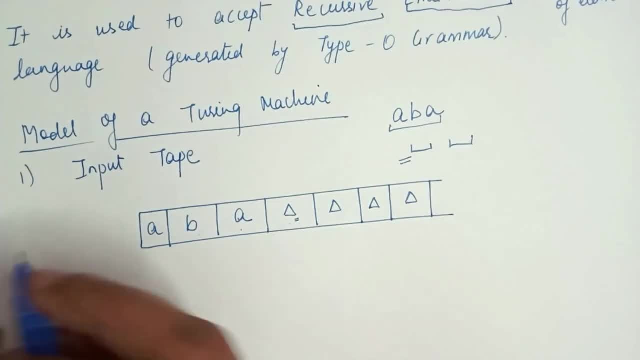 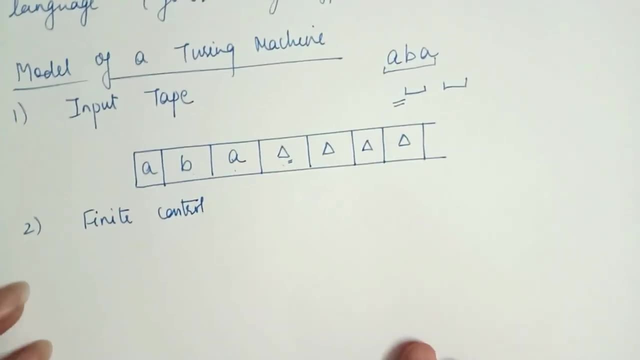 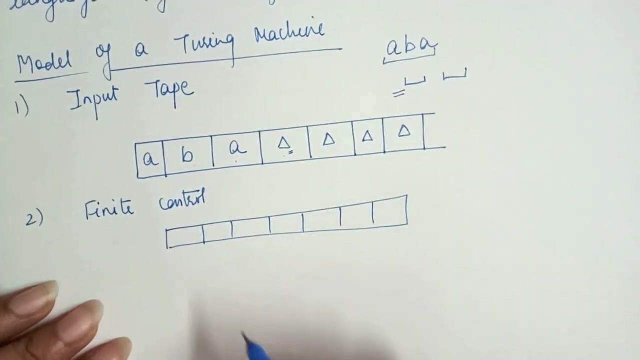 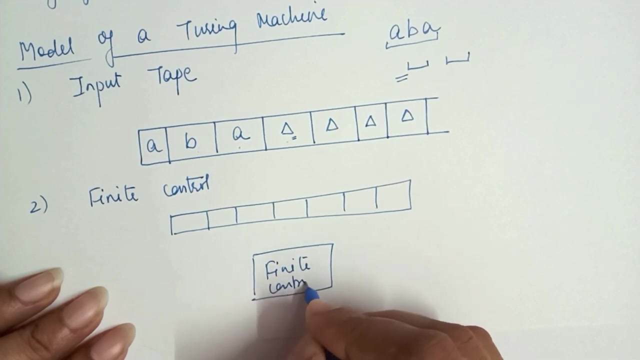 The second component of the Turing machine is: is that is finite control. So what is finite control? Suppose this is our input tape in which we have infinite number of cells, and if this is a finite control, and this finite control suppose map to this cell of the input tape. So this: 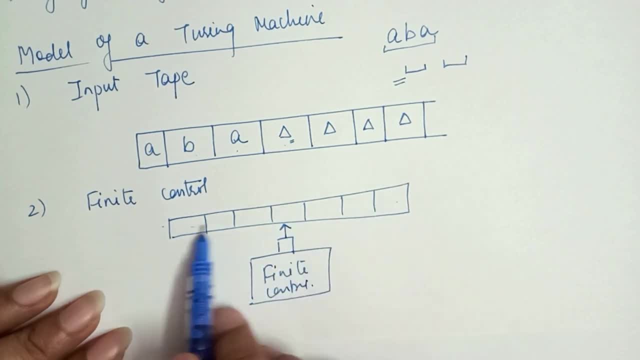 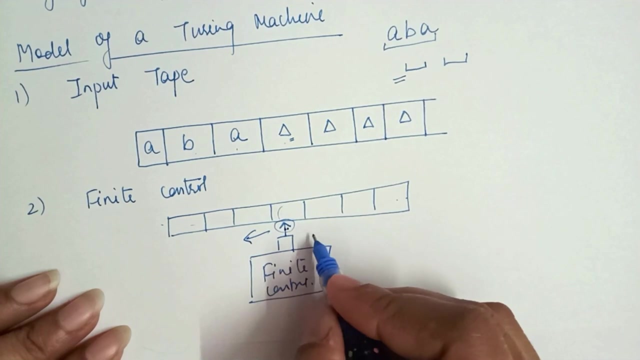 infinite, this finite control, and the tape, tape head. this is called tape head. Okay so, the finite control and the tape head, which is responsible for reading the current, current input symbol, and the tape head can be moved, either moved to the left or it can. 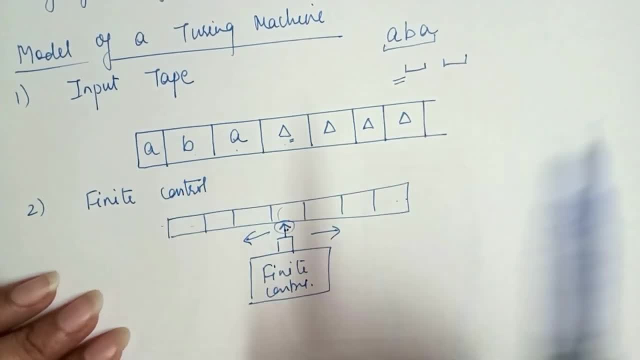 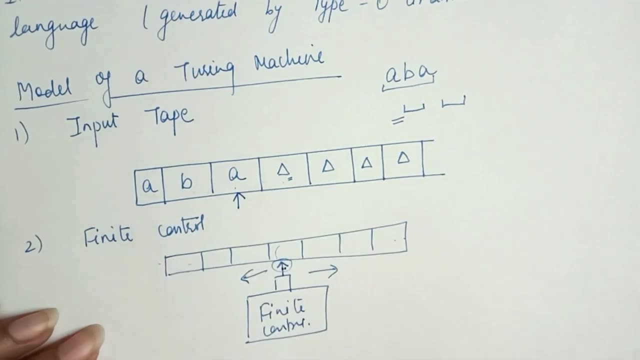 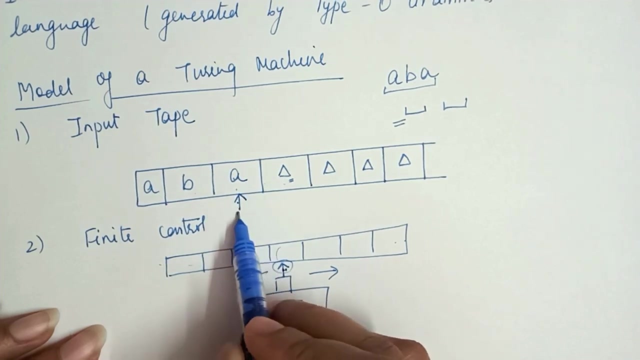 either move to the right. This means that, suppose, if we are having a string like ABA and if we place this ABA like this, and if this input head, or you can say tape head, is positioned to this cell, this means that it currently read this character A and which is also responsible for the finite. 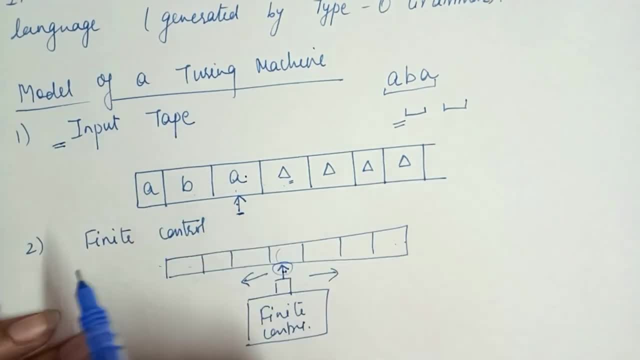 control. Okay, so the first component is input tape, the second is finite control and the second is finite control. So this is the finite control and the second is finite control. So this is the finite control and the second is finite control and the second is finite control. 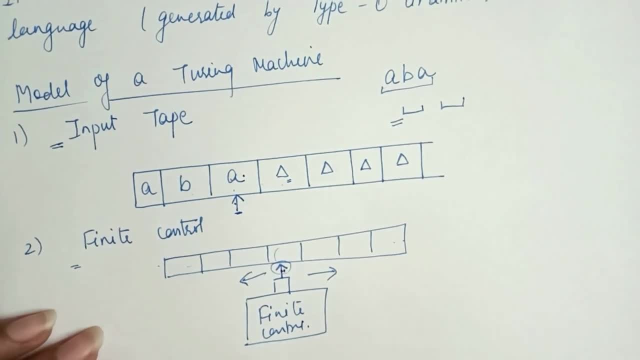 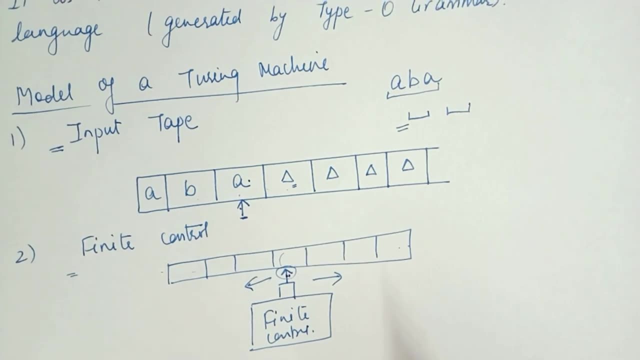 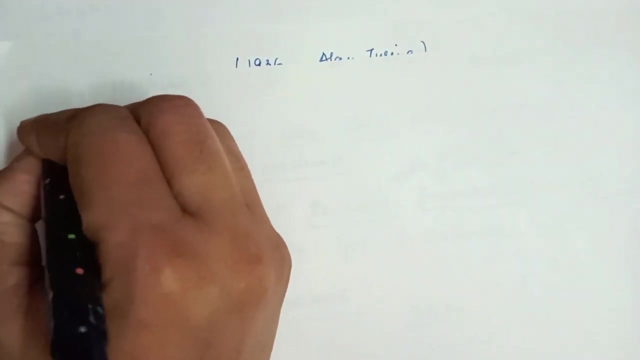 And a finite set of states through which machine has to undergo and finite set of symbols, called external symbols, which are used in building the logic of a Turing machine. So now we discuss that, how we represent a Turing machine. So for the representation, for the representation of Turing, 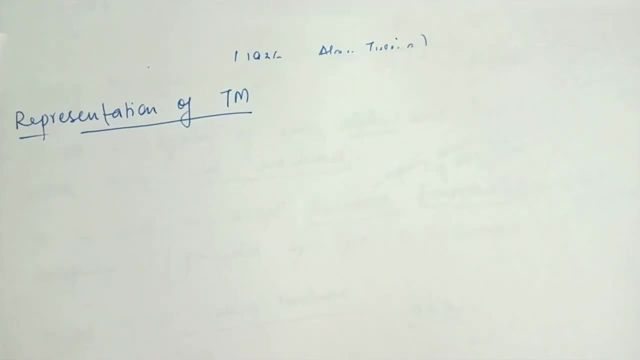 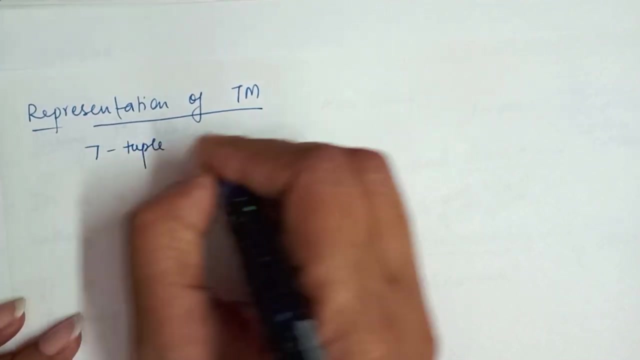 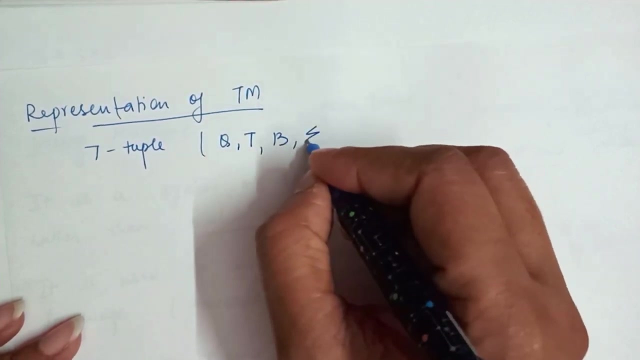 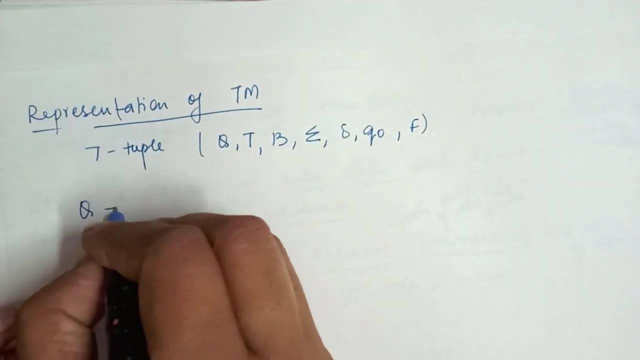 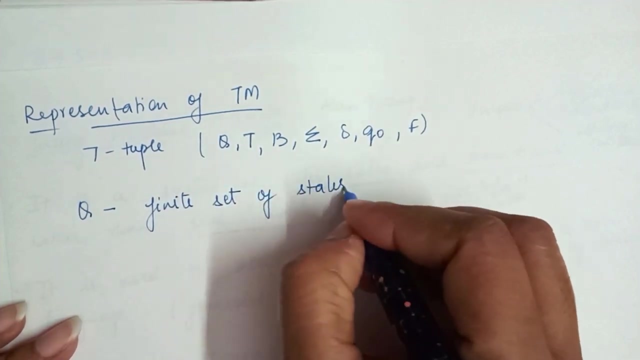 machine, in short, the Turing machine, will be represented by Tm. So, for the representation, it is represented by 7 tuple. and what are the 7 tuples are 7 tuples are Q, T, B, sigma, transition function, Q0 and F. Now, what is Q? Q is finite set of states. Q can be represented as finite set of state. 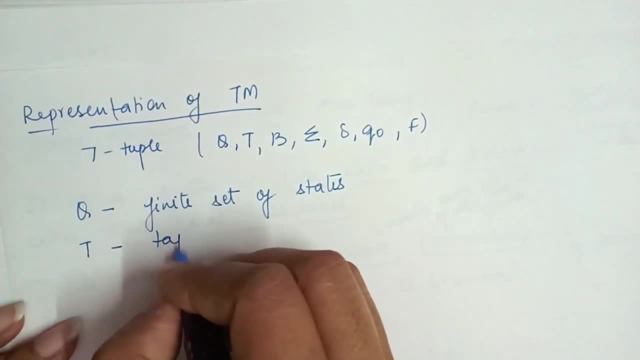 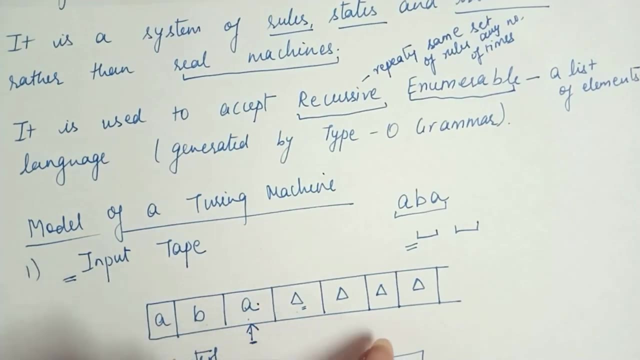 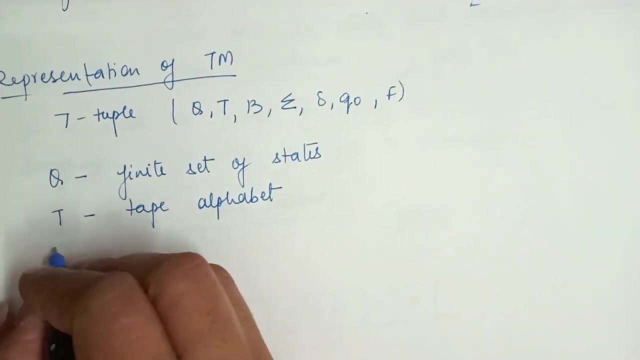 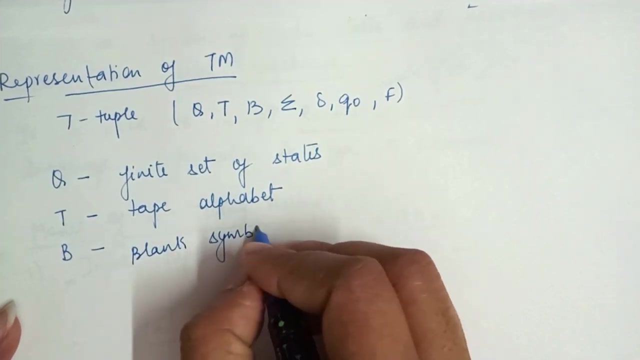 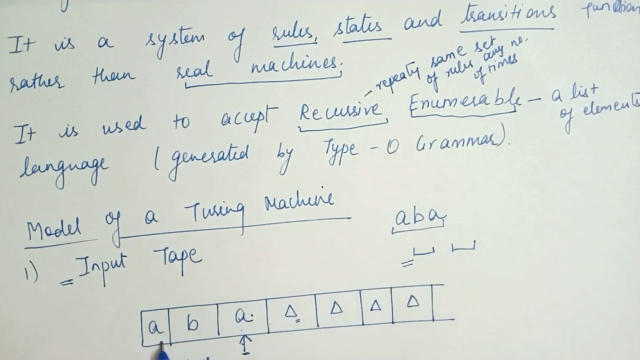 This T represent as tape alphabet. tape alphabet means the input symbols that are placed in this input tape. So this T is input alphabet, which are symbols are written on the tape. Now B, capital, B, is blank symbol. blank symbol that will be represented by delta means the input string that we are having. So we place this input. 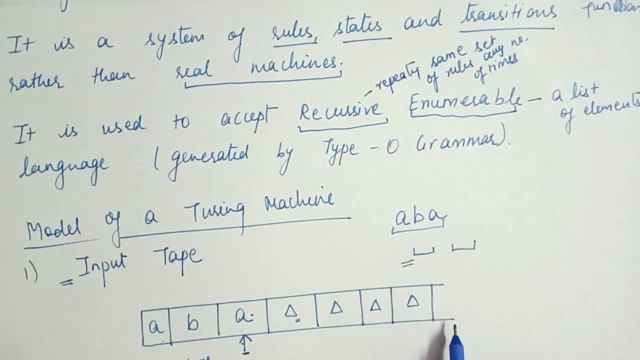 one by one in one set. So this is the input string that we are having. So we place this input one by one in one set And the remaining empty tape will be represented by is all we can say. it is filled by the blank. 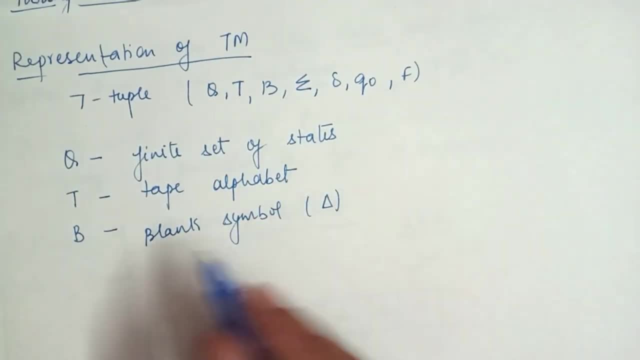 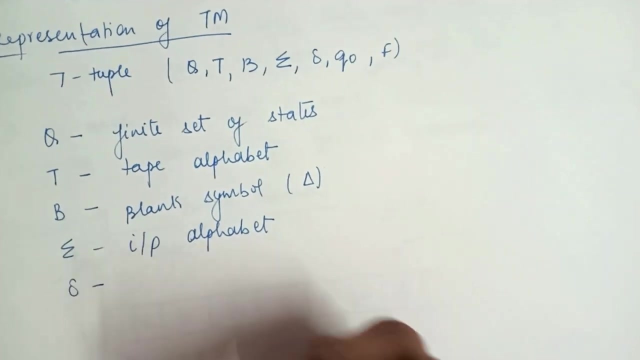 symbol that is called del. So B is blank symbol. Now sigma is input alphabet, input alphabet and symbols which are a part of the input alphabets. Then transition function. So this transition function which maps, like this, Q into T. 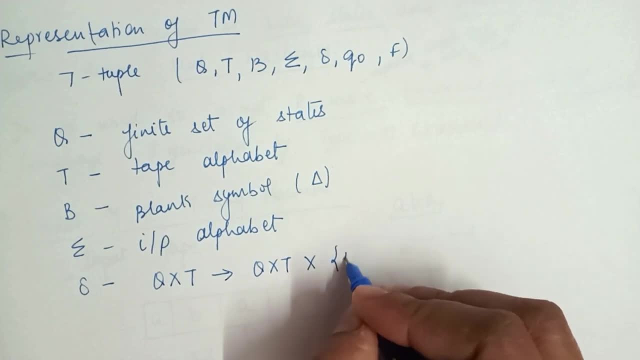 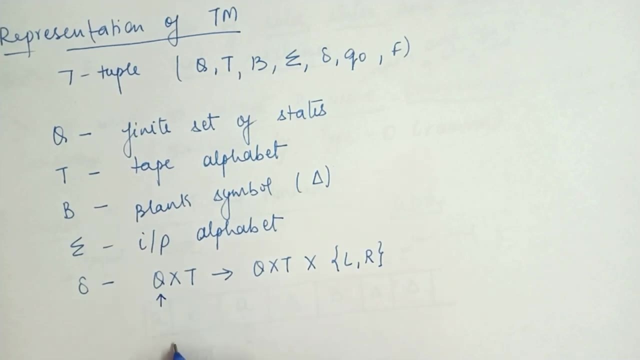 it gives Q into T, into either L or R. What does it mean? This means that, depending upon the current state- okay, depending upon the present state and the present tape symbol or present tape alphabet which is pointed by the head pointer, it will move to the next. it will move to the next state. 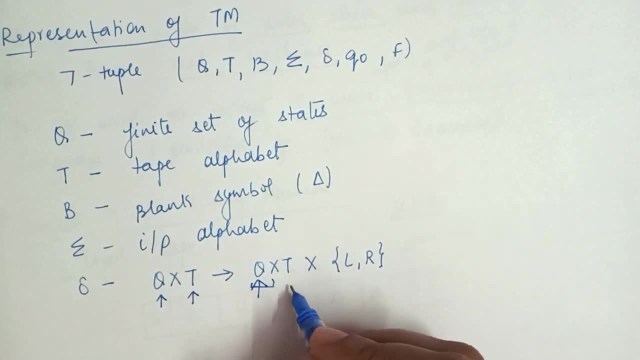 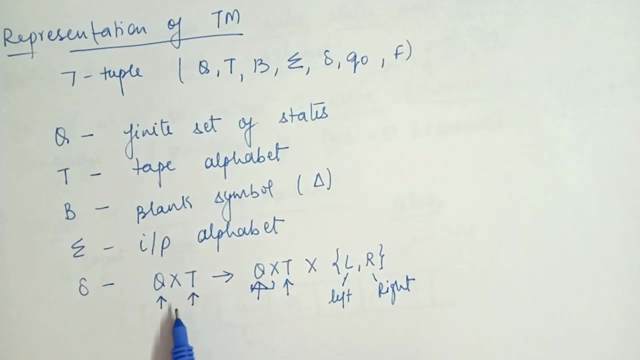 this is the next state, okay, and it changed the tape symbol- it may or may not be changed- and move the head pointer either to the left of the tape or R stands for the right of the tape. So this transition function can be defined as that, depending upon the present state and the 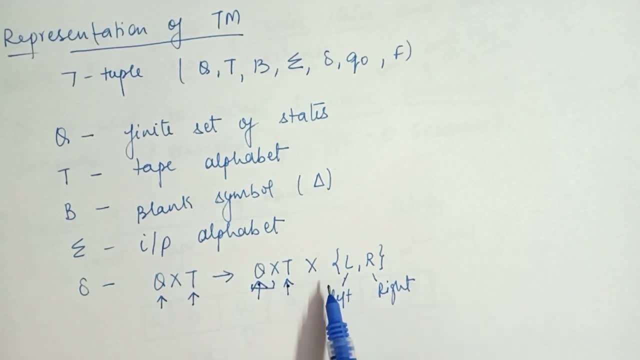 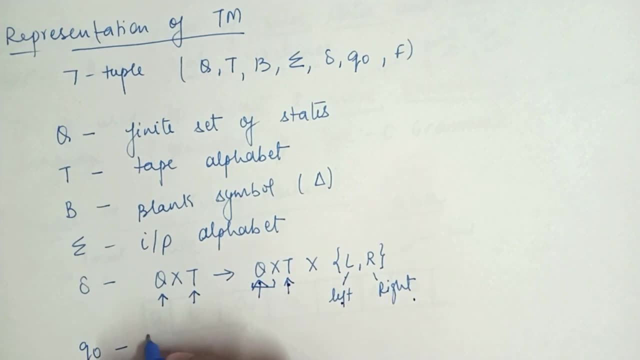 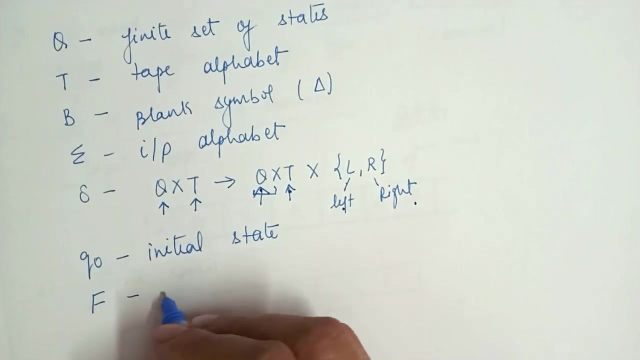 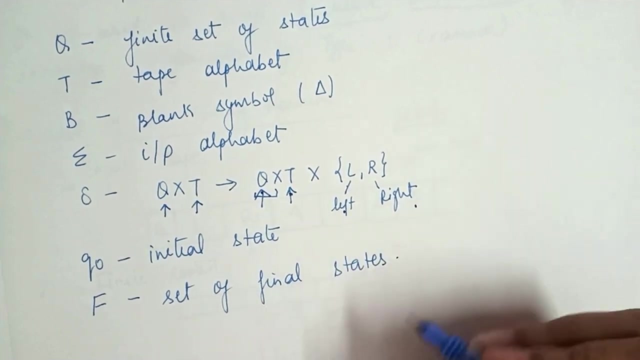 or may not, change the tape symbol and move the head pointer either to the left or the right. okay, Now this. q0 is initial state, initial state, and f is final. f is set of final states, set of final state and, if any state, if any state of f is reached, their input symbol is: 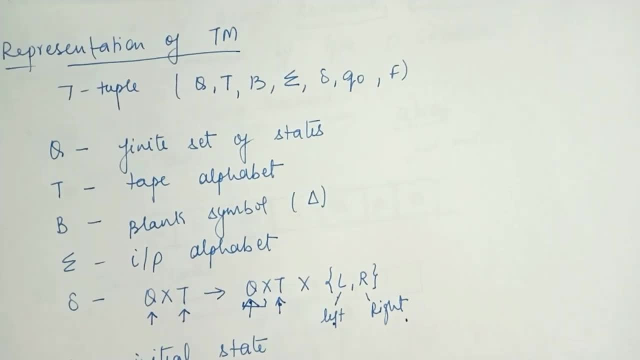 accepted. So the Turing machine can be represented by these seven, with the help of these seven tuple. and this is the basics about the Turing machine. So what is the history of the Turing machine, what are the basic models, or you can say what are the components or how. 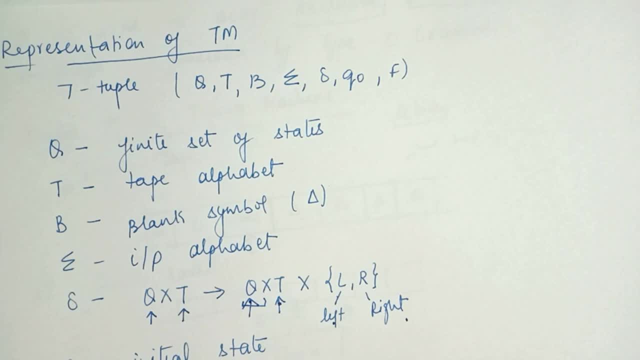 they represent a Turing machine with the help of some tuple. So I hope you understood this. and still, if you have any query, then you can ask in our comment section and keep watching our video. and in my next video I am going to discuss the language which are accepted by a Turing machine. 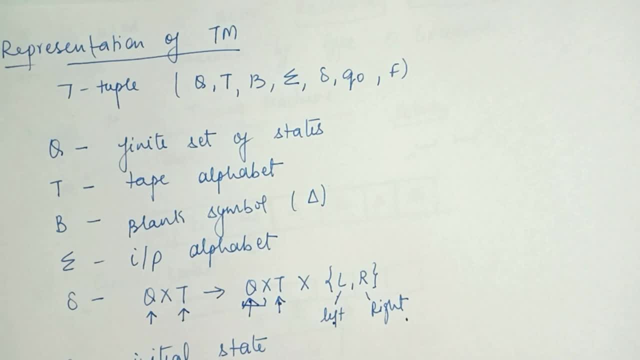 with the help of some tuple. So keep watching our video. Thank you so much.